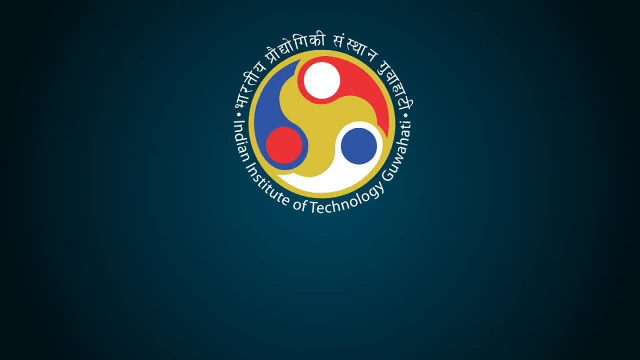 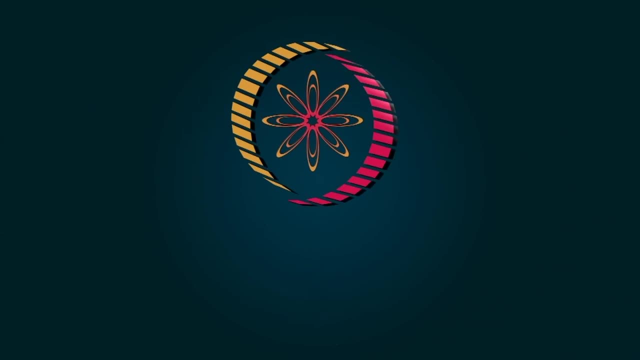 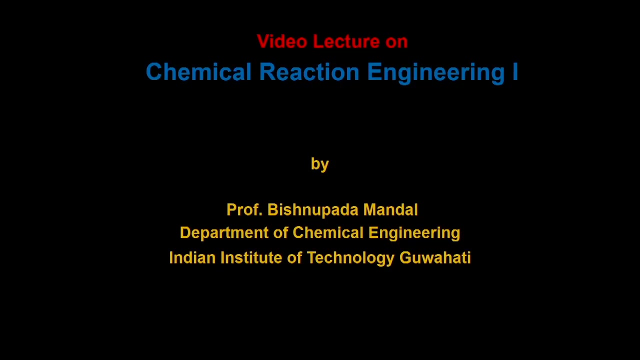 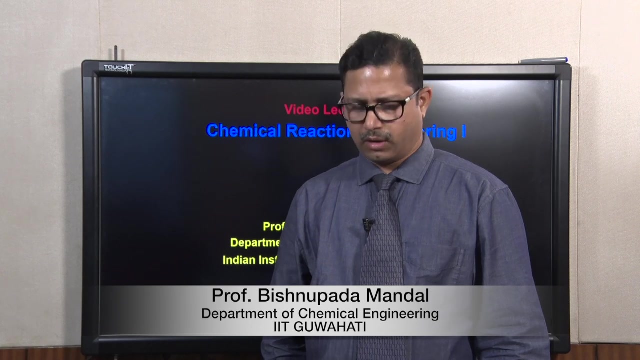 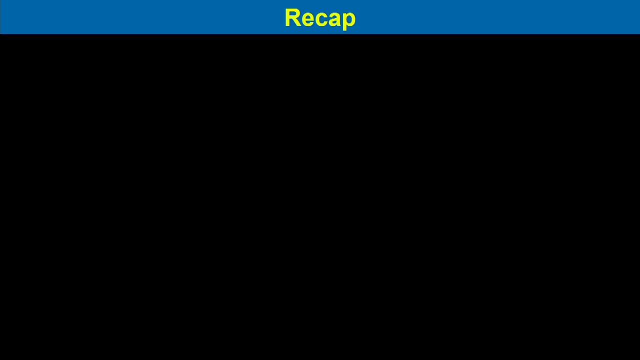 Welcome to the second lecture of module 2 on chemical reaction engineering 1.. Before going to this lecture, let us have small recap on our previous lecture. In our previous lecture we have covered few important topic, that is, introduction to the chemical reaction engineering 1.. Then we considered different reactions and there are 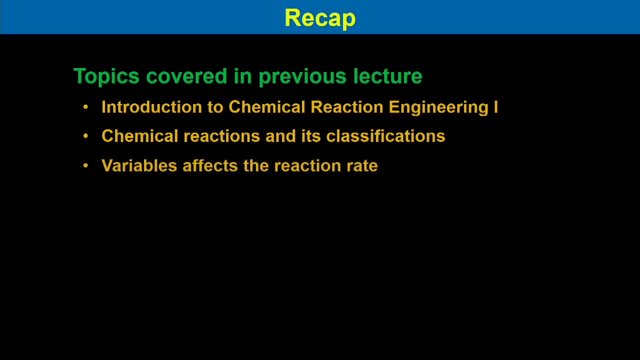 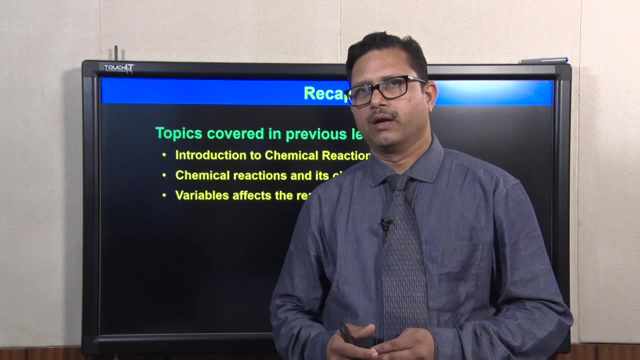 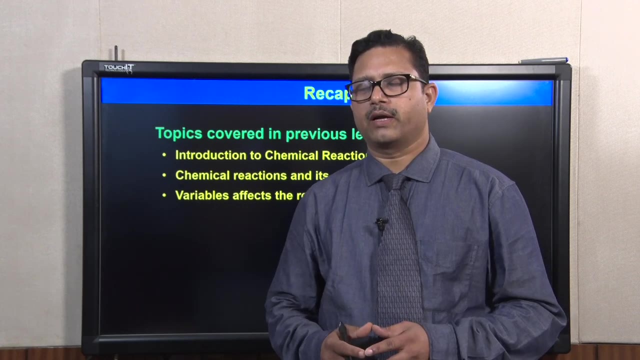 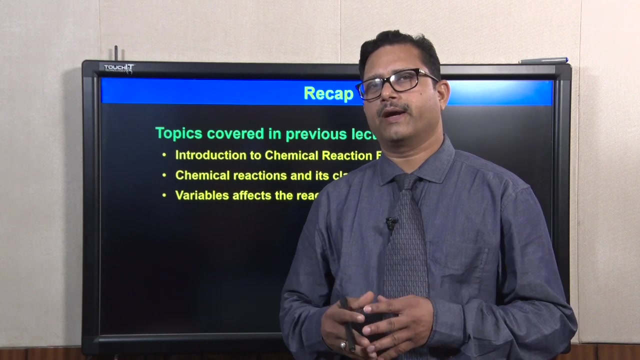 classifications, different variables. that affects the reaction rates. Here we have considered for homogeneous reactions and for heterogeneous reactions. what are the variables that influence the rate of chemical reactions? Like in case of homogeneous reactions, we saw that the temperature, concentration and temperature. And these are the major variables which influence the rate of chemical reactions. In case of heterogeneous reactions, we have seen that the parameters, which are temperature, pressure and composition. in addition to that, we have seen the heat and mass transfer effects also affects the rate of chemical reactions. 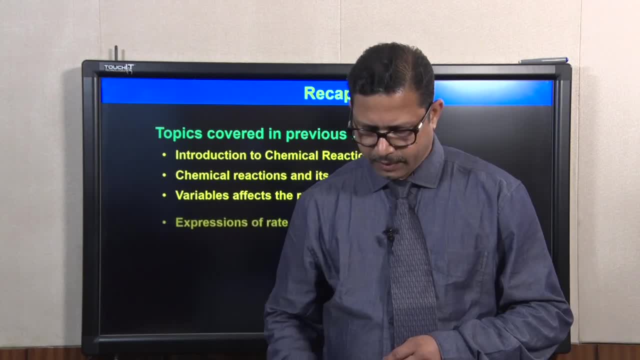 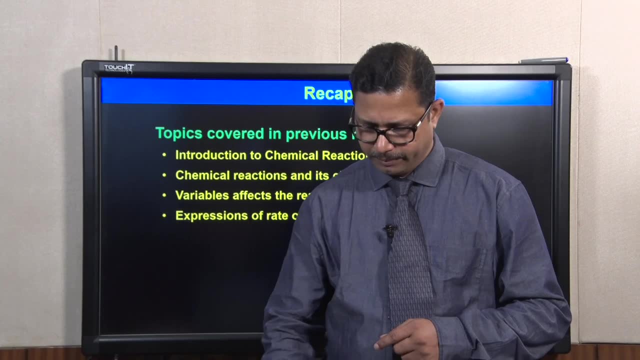 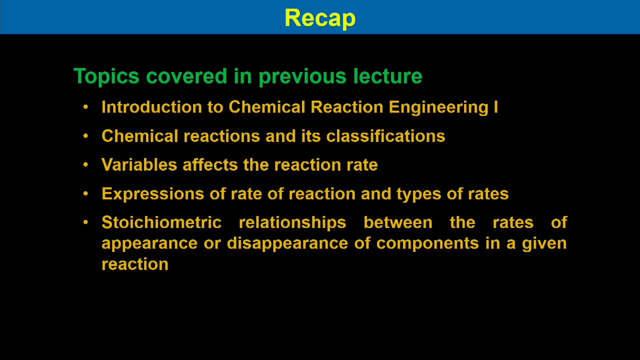 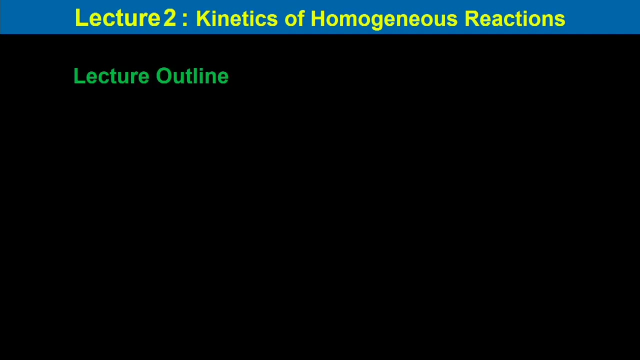 reaction. Then we have different types of rates and we have seen the correlations among them and also we have seen that the stoichiometric relationship between the rates of appearance or disappearance of the component in a given reaction. So in this lecture we will consider kinetics of homogeneous reactions. So the brief outline. 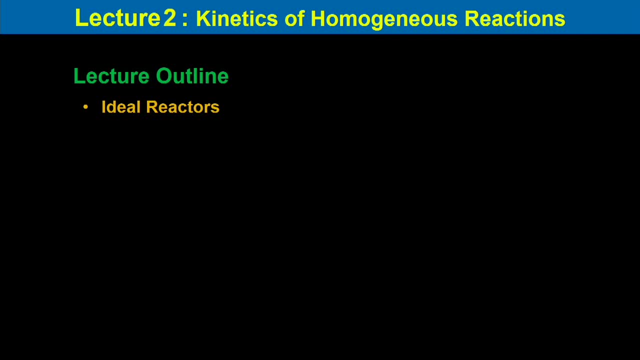 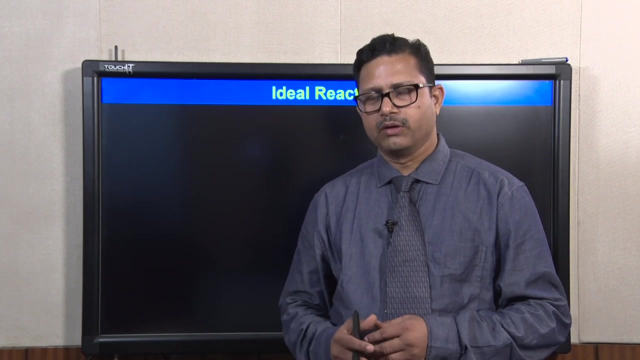 of this lecture would be the ideal reactors, then reaction rate rate constants and its unit. then we will discuss the elementary and non-elementary reactions, reaction order and rate law, molecularity and deriving rate law from different elementary reactions. So let us start with ideal reactors. In general, there are three ideal reactors of which we 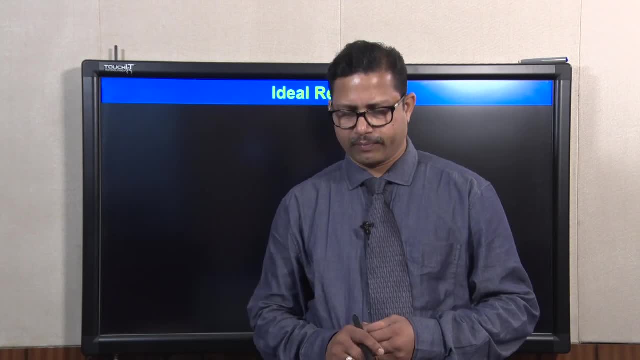 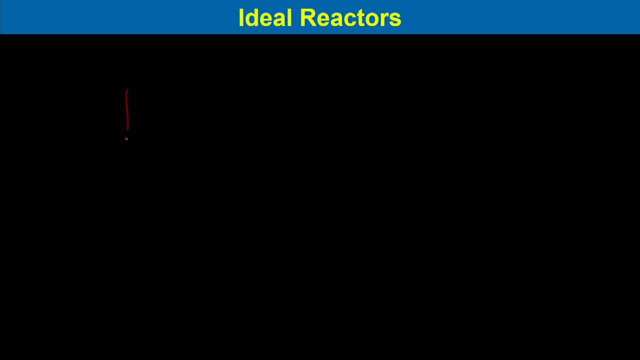 generally considered in chemical reaction engineering. These three ideal reactors are: one of them is the badge reactor. So you have a tank and you have a stirrer or impeller fitted into it Here. initially you have put some raw materials inside the reactor and 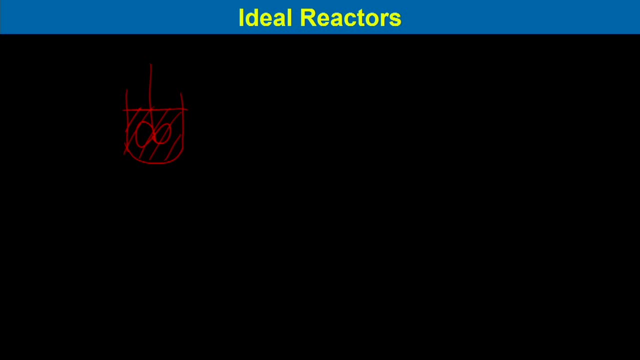 there is, then you close it. So there is no inlet or outlet for these reactors, and you can stir it for a certain period of time and then you can take out the products. So this is known as badge reactor, In this case your composition- everywhere. 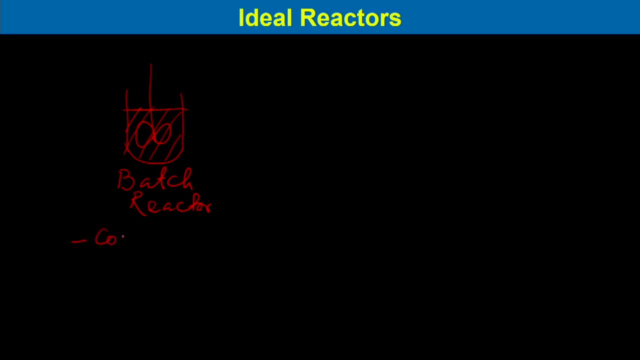 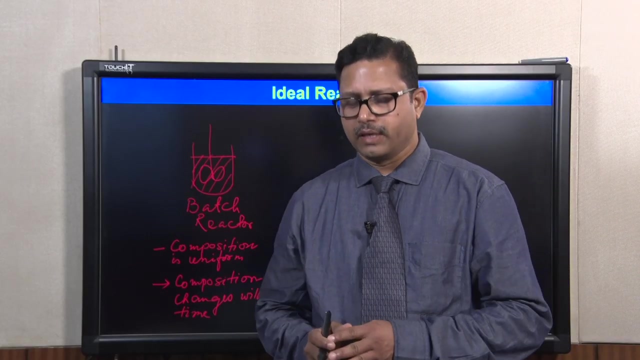 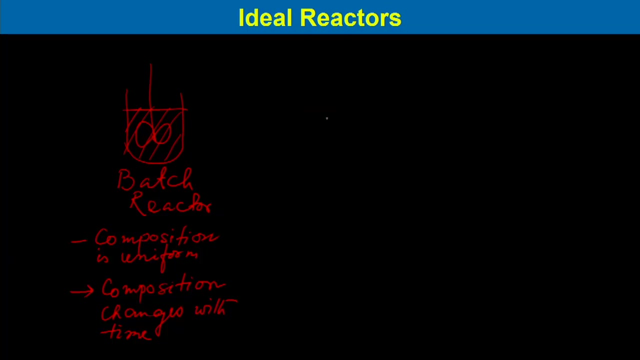 is uniform. So composition is uniform everywhere inside the reactor. but the composition changes with time. 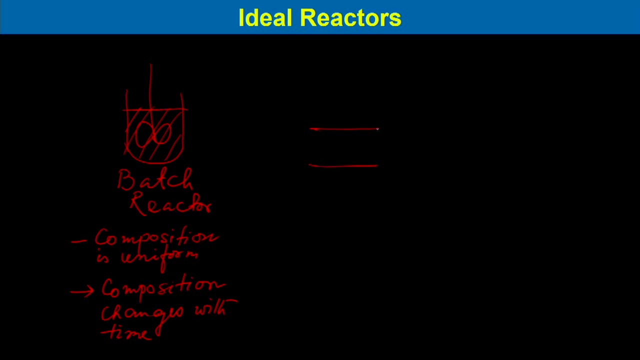 You can think of a simple cylindrical. 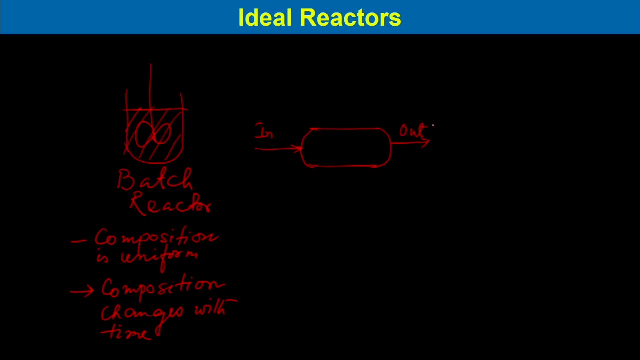 pipe. so the fluid through which is enters and it flows through and there is no overtaking of the fluid which is behind. behind that means there is no bag mixing in this case. that is why we call it plug flow. So this is plug flow reactor. So in this case no axial mixing, that is, there is no overtaking. 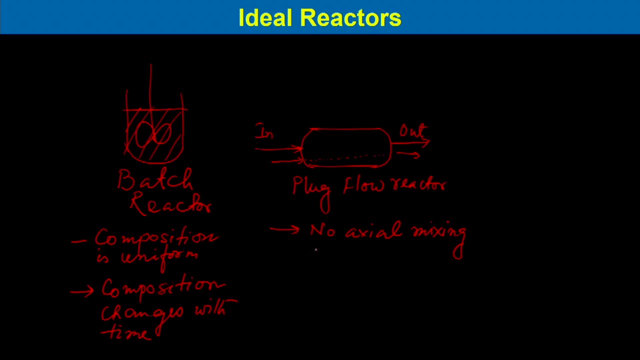 of the fluid. So in this case it is not a problem. So we can say that the liquid is moving through the plates, Moving through the plates reactor. The other idealized reactor is continuous start tank reactor. So it is like a tank fitted with impeller and you have fit in and 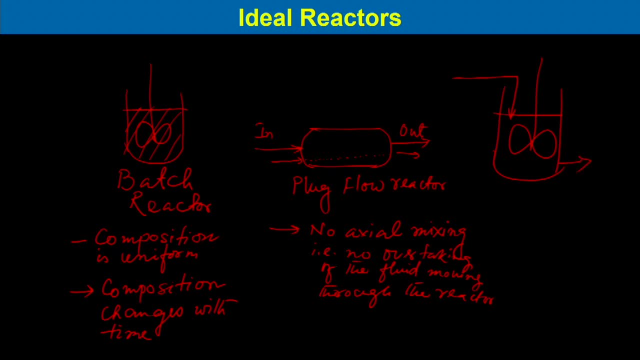 you have product out, So raw materials or the reactants, in to the reactor, mixed it with an impeller and then you have a output. So all these are. these two are flow reactors. So this is in and this is out. 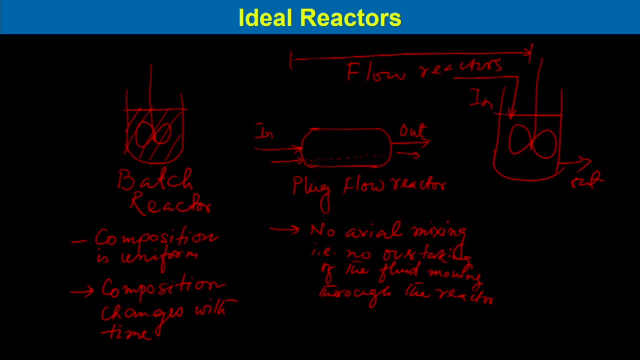 So in this case it is: the mixing is uniform, homogeneous and at steady state. the composition inside the reactor as well as at outside are same, So the composition uniform mixing. in this case composition is uniform at inside, the inside, the 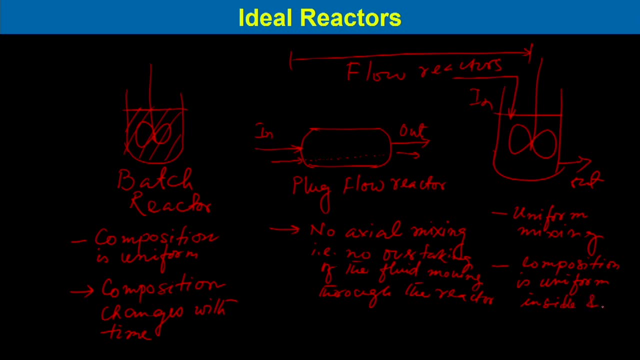 reactor and exit of the reactor. So the composition should be same inside the reactor as well as which is coming out from the reactor. So these are the three idealized reactors. We will consider more details on it while designing. designing of the reactor. Now, reaction rate and the rate constants. 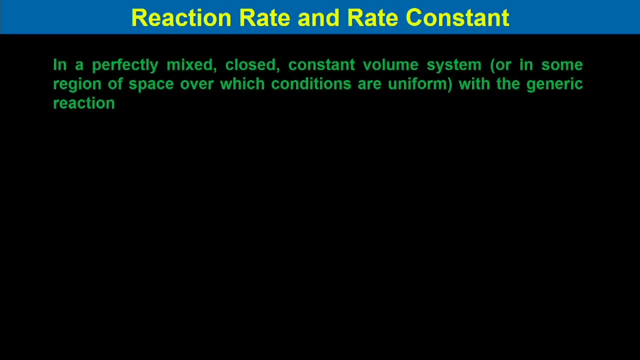 So in a perfectly mixed, closed and constant volume system, or in some region of the space over which the conditions are uniform, we can write the generic correlations or the reaction. that is a eldest of the future. 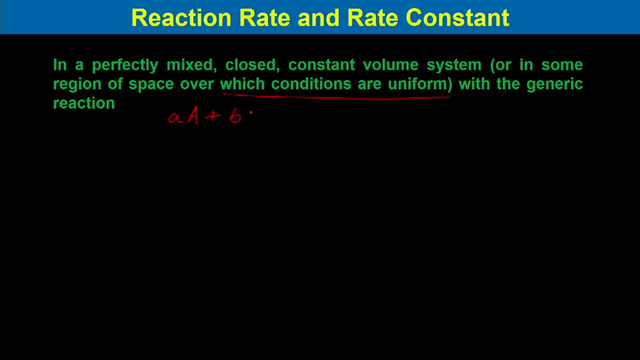 A plus B, B, producing C, C plus D, D. So we can write the rate of disappearance of A as minus R, A would be equal to minus 1 by V, d, N, A, d, t, So which is equal to moles of A. disappearing. 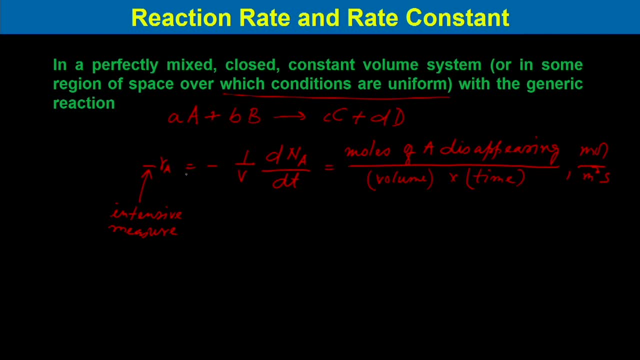 That means the concentration is decreasing of the reactants. So that is why the minus sign indicates the disappearance. Now reaction rate. for this reactions we can write: R would be equal to minus. R A divided by A is equal to minus. 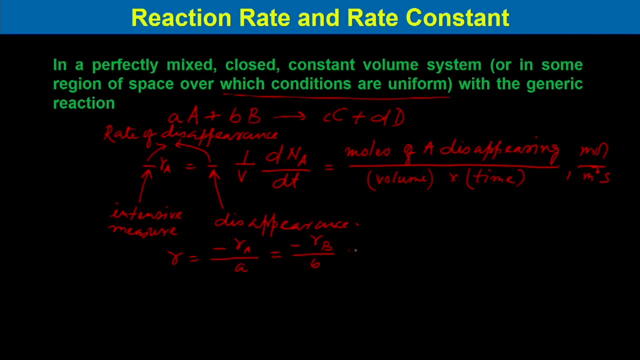 R B divided by B, which would be equal to R C divided by C, which would be equal to R D divided by D. or we can write this: R is equal to minus 1 by A d C, A d t minus 1 by A d C. 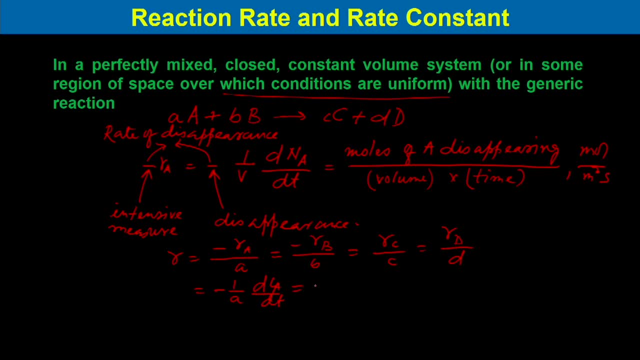 A d t, Which is equal to minus 1 by B d C, B d t, which is equal to 1 by C d C, C d t, which is equal to 1 by D d C, D d t. The coefficient, as you can see, minus A d C, B d t, minus 1 by B d C. 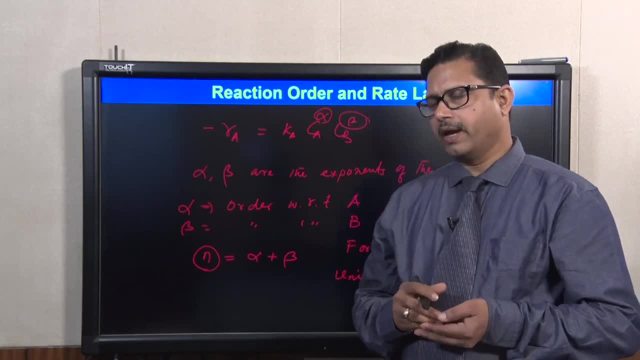 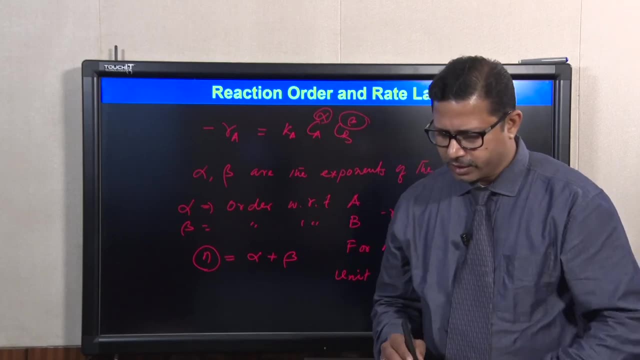 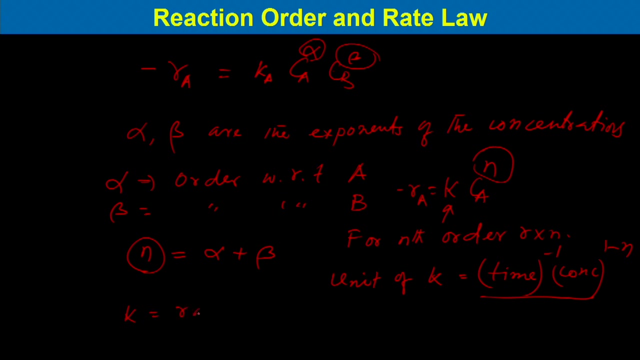 at a particular temperature. but essentially K is a function of temperature. So the better term to use for K is the rate coefficient in instead of rate constant, coefficient instead of rate constant. So K we can call rate coefficient. Now, if we 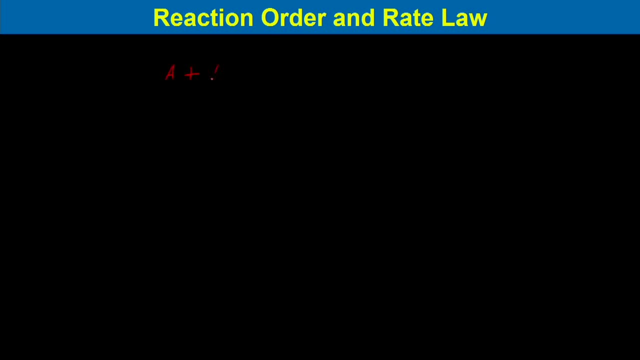 considered a general reaction A plus B to C and the rate law we can write: rate is equal to K, C, A to the power alpha and C, B to the power beta. and this alpha and beta, they are determined. So we can write experimentally: For example, if we consider 2, N, 2 O, 5, gas, it converted. 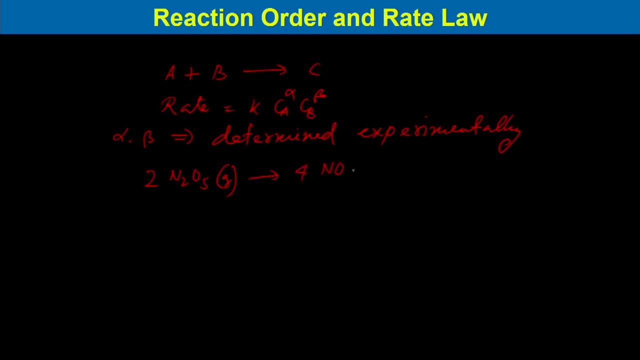 to 4 NO nitric oxide gas, So N 2 O 5 gas, So N 2 O 5 gas, So N 2 O 5 gas plus oxygen gas, and the rate is given as K concentration of N 2 O 5. that. 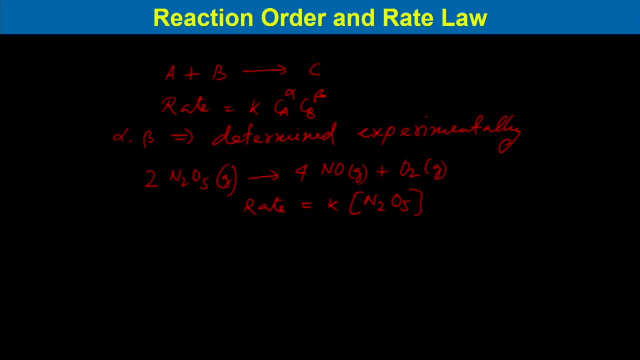 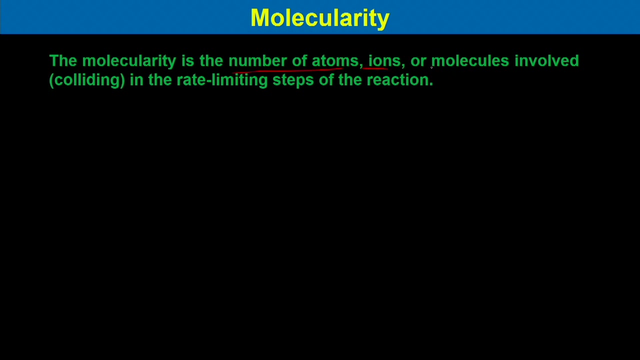 is, the reaction is first order. So this is another important topic, which is molecularity of the reaction. The molecularity is defined is the number of atoms or ions or molecules involved in the rate limiting steps of the reaction, Based on the number of molecules involved for a rate limiting. 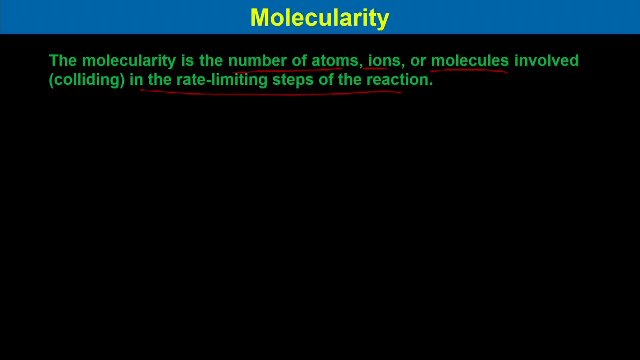 steps. we can define it as unimolecular, bimolecular and trimolecular and so on, But the unimolecular and bimolecular reactions are common, but termolecular reactions are very rare. One common example of unimolecular reaction is the conversion of the uranium. 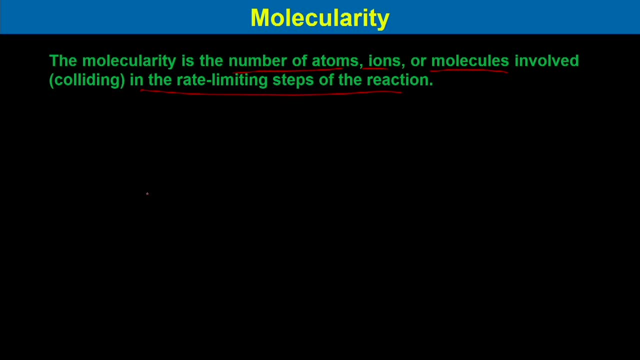 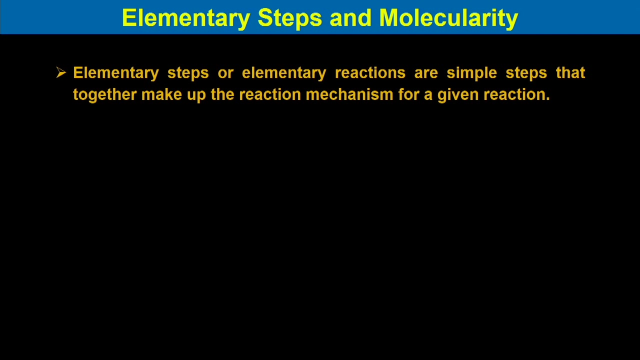 To thorium and helium. So this is the reactions of radioactive decay And this is the reactions in spontaneous in nature. So elementary steps or elementary reactions are simple steps that together make up the 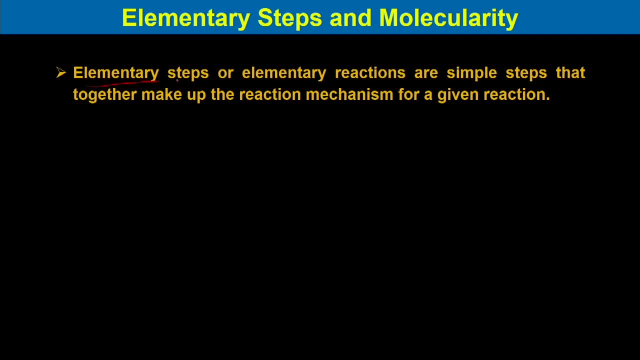 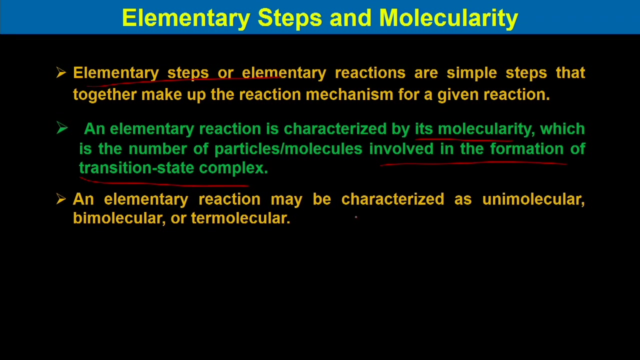 reaction mechanism for a given reactions. An elementary reactions is characterized by its molecularity, which is the number of molecules or particles involved in the formation of the transition state. complex And elementary reactions may be characterized as unimolecular, bimolecular and termolecular. 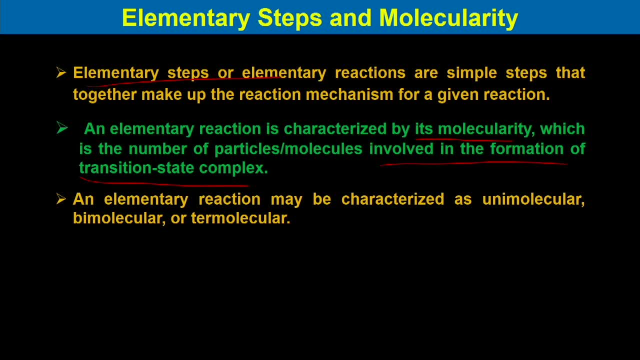 which I have explained before. So the, if we consider elementary reactions, then it would be easy to find out the rate of the reaction and the molecularity will be based on the elementary steps of the reaction: Unimolecular and bimolecular reactions, as I said, it is the most common in the processes. 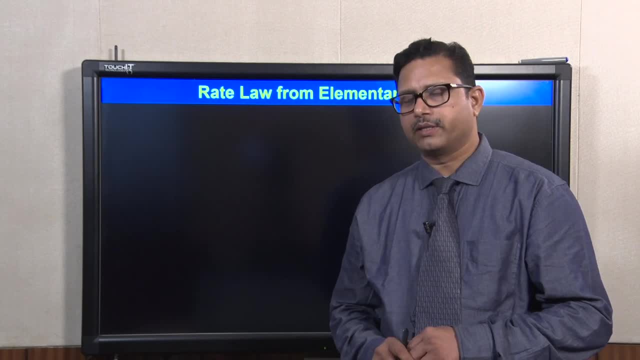 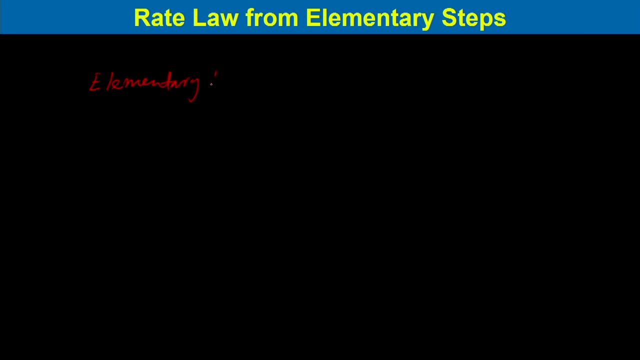 Now you will consider rate law from elementary steps. So if we consider elementary reaction, say A 2 product, then we call the molecularity. So we consider the molecularity as unimolecular and the rate law if we can obtain from here. 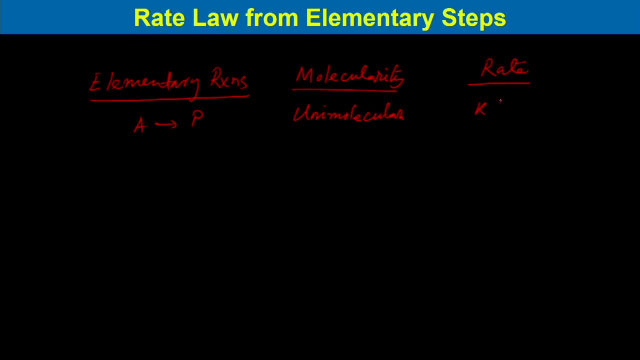 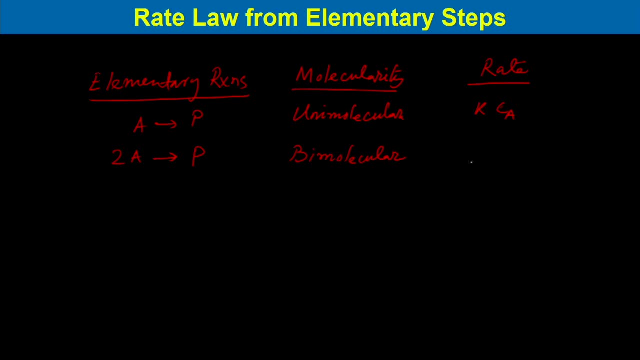 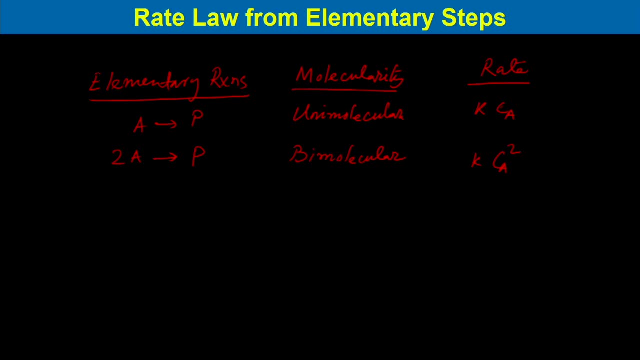 So this is bimolecular reaction. Now if A plus B produce P, this is also 2 different reactants reacts together, producing product P. This is also bimolecular reaction. and the rate we can write K into C, A, C, B And 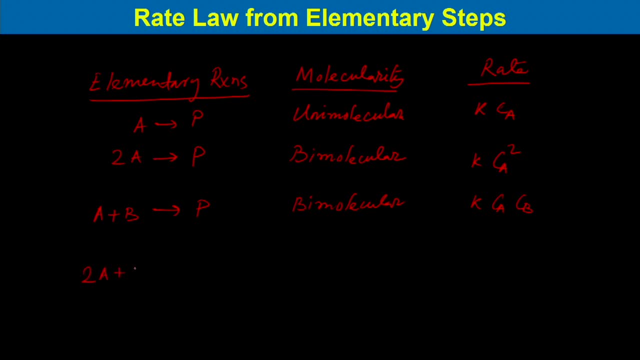 another one. if twice A reacts with B and forms product, then we can write till this reaction as termolecular and the rate would be K into C A to the power, 2 into C B. So, as we said, the termolecular reactions are very rare. 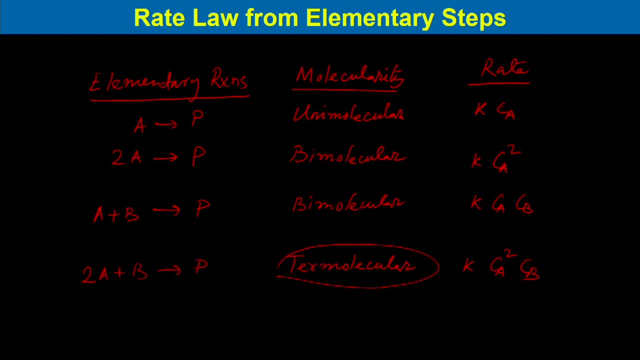 One example of termolecular reactions is assumed to happen for the conversion of oxygen to ozone. So oxygen reacts with nitrogen and it forms O 3 plus O plus the activated complex of nitrogen species. So this reaction is considered as termolecular reactions, but in general the termolecular 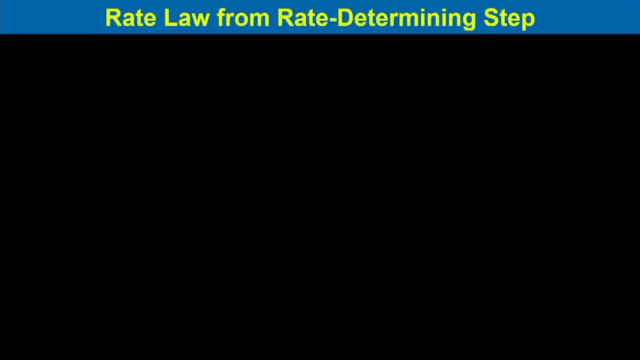 reactions are very rare. Now we will consider rate law from rate determining steps, How to obtain the rate equation or the rate law from the rate determining step If a proposed mechanism consists of more than one elementary steps. in that case, the slowest steps- or there are steps where the rate is the slowest of the overall reactions- can be. 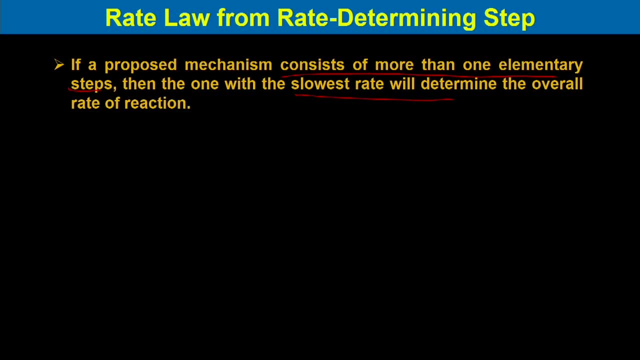 obtained Ok reactions is considered as the rate determining steps. So it is called the rate determining steps, which step represents the rate law of the overall reaction, Like if we consider a reactions NO2 plus CO reacting and then forming NO plus carbon dioxide. 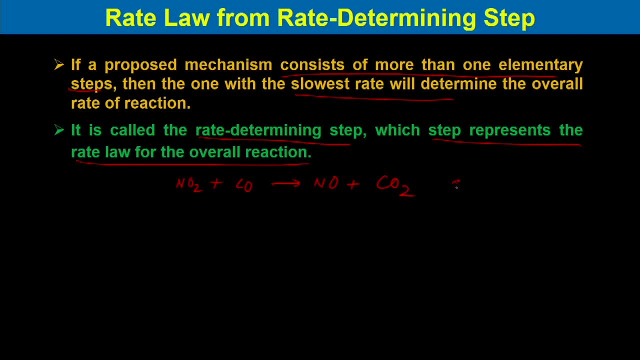 and the reactions happen in a single step. So in that case we can write the rate is equal to K into concentration of NO2, into concentration of CO. However, the experimental measurements shows that The rate is actually K into concentration of NO2 square. So now, if we propose this: 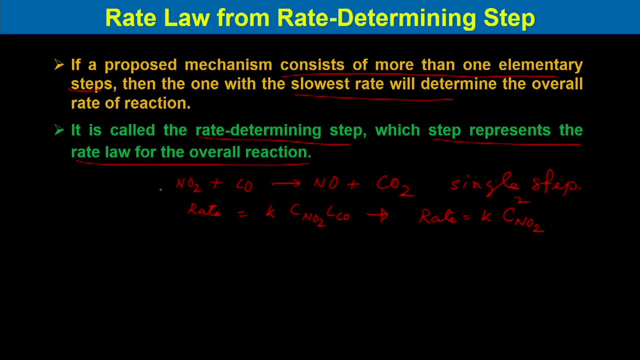 step into 2 elementary steps. this reactions. if we propose into 2 elementary steps, we can write: Step 1. Step 4. Step 5. Step 6. Step 7. Step 8. Step 9. Step 10. Step 11. Step. 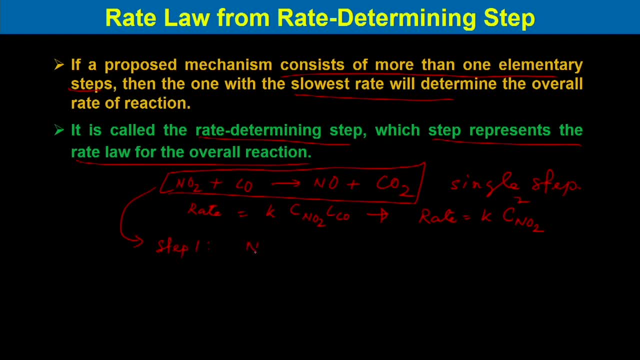 NO 2 reacts with NO 2, forming NO 3 plus NO, with a rate constant k: 1.. And step 2, NO 3 reacts with CO, forming CO 2 plus NO. So this reaction is actually slow and this reaction is fast. 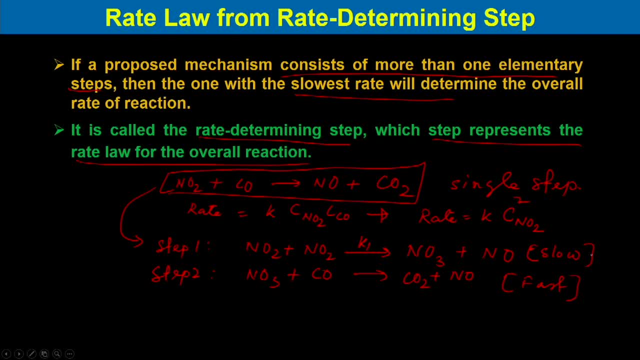 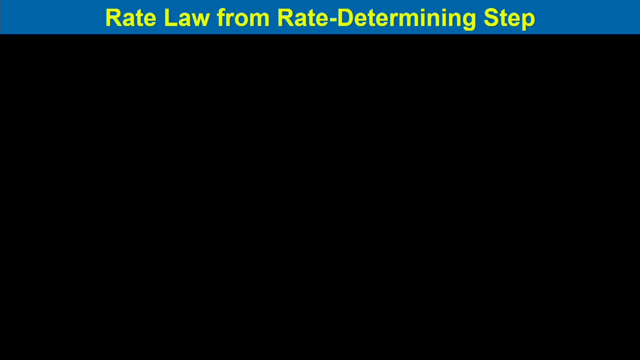 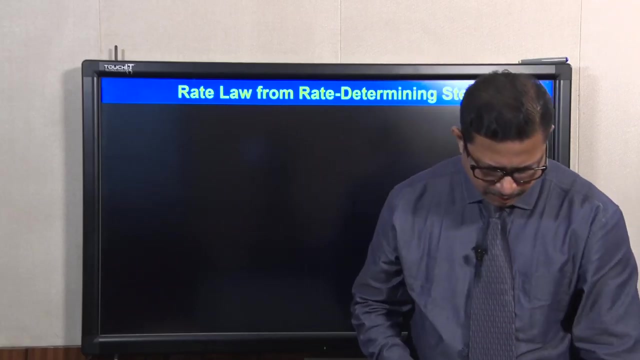 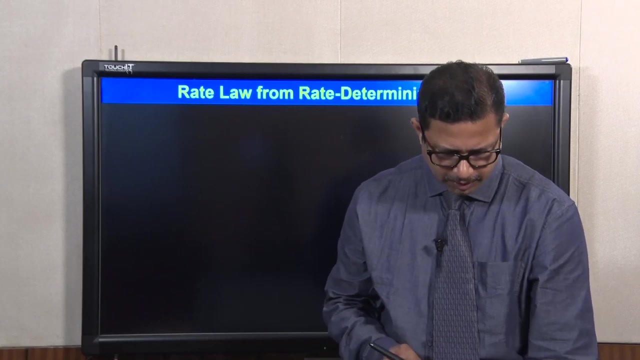 So this is the rate determination Determining steps. So from here we can write: the rate is equal to k into CNO 2 square. So, as we have said, the overall reaction rate must be determined experimentally or the rate law must be obtained from the experimental measurements. 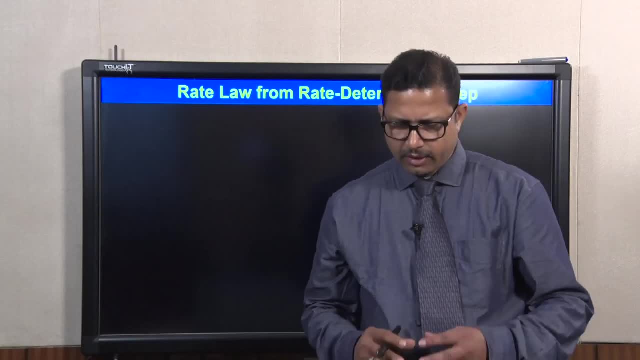 And if the rate law is obtained from the experimental measurements and if the reaction rate must be determined experimentally or the rate law must be obtained from the experimental measurements. and if the rate law is obtained from the experimental measurements and if there is elementary reaction, then the rate equations can be obtained directly from the. 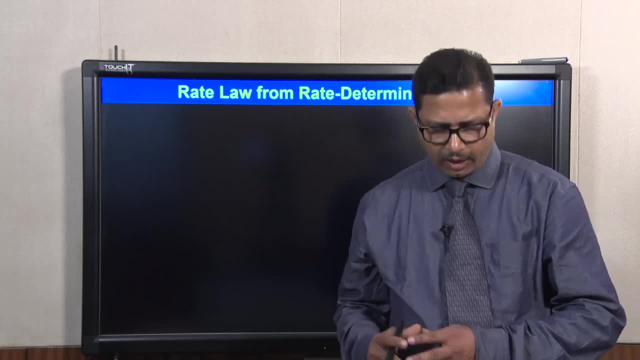 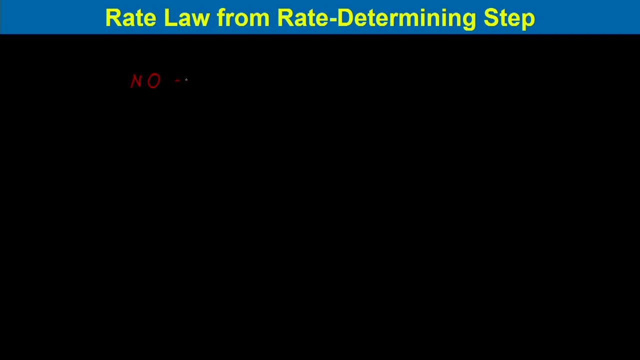 elementary reaction or from the molecularity of the reaction, Like for following examples, it forms, and we can write the rate minus C, N, 2 square. So if the rate is r 1 is k, C, N, o into C concentration of ozone. Similarly, if N 2 O, 5 decomposes, 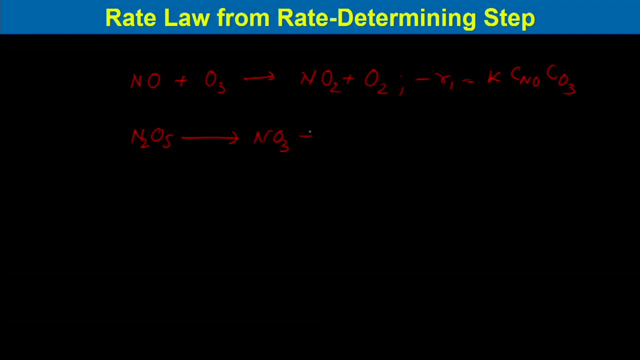 and forming NO 3 plus NO 2, we can write as k into concentration of ozone, So here also we can write the rate of the reaction to the reaction. So from the experimental measurements we have found that the rate of the reaction to 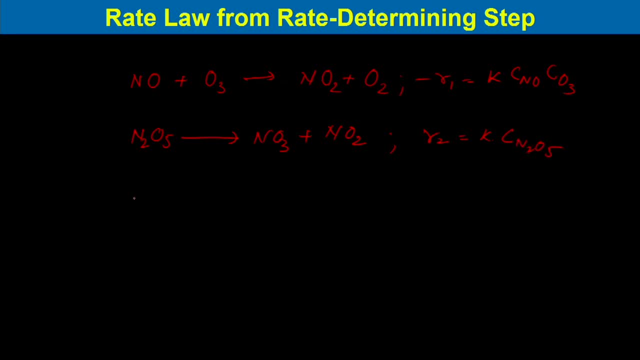 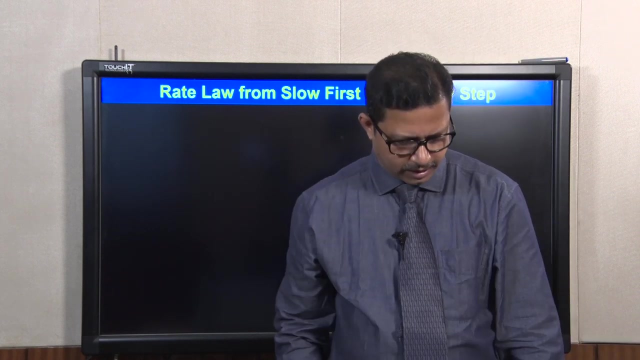 of N 2 O, 5.. Similarly, bromine plus nitric oxide reacts and form O N B R 2. the rate can be written as K into concentration of bromine and concentration of N? O. Now we can also obtain the rate law from the slow, fast elementary steps, like if we 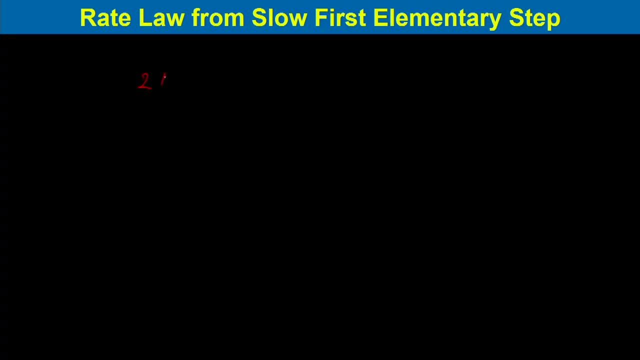 consider the reaction twice: N O N O 2, N O 2, N O 3, N O 4, N O 5, N O 6, N O 7, N O 8, plus fluorine it forms twice N O 2 F and the rate we can write K into concentration. 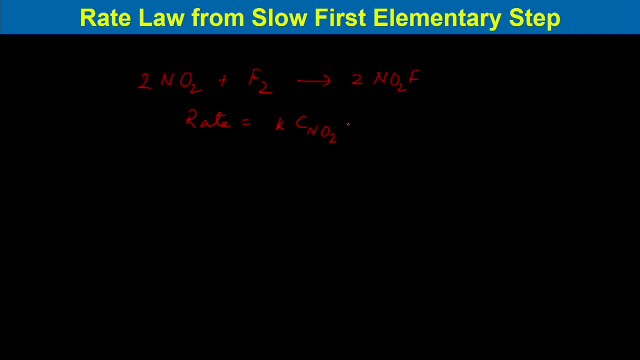 of N O 2 into concentration of fluorine. The A proposed mechanism for this we can write: N O 2 reacts with fluorine, form N O 2 F plus F. N O 2 F can form N O 2 F and the overall reaction is like this: 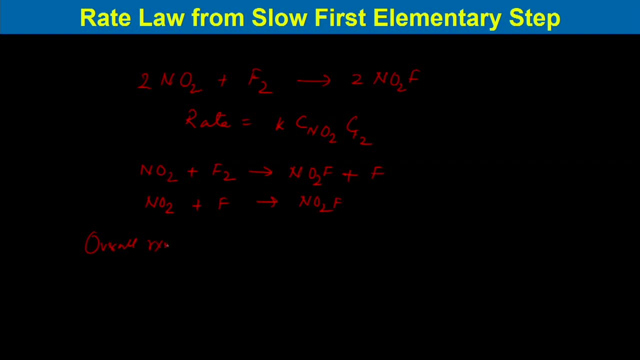 So if we sum it up, so this will cancelled out and we will have twice N O 2 plus F 2, forming twice N O 2 F. So this is the first step And it is considered as slow and rate determining. and this is the second step and considered 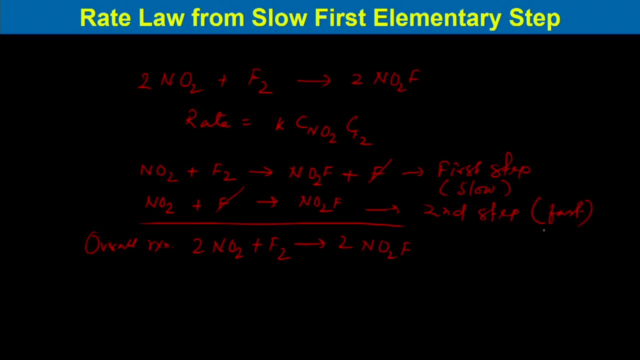 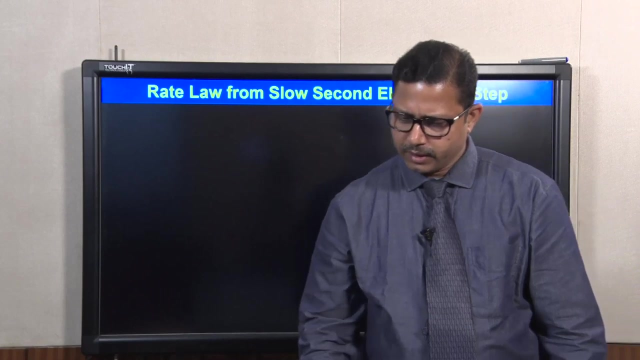 as fast, So the, So the rate of reaction. for this we can write K 1, say this is K 1, concentration of N O 2 and concentration of fluorine. Now, rate law can also be obtained from the second step, which is slow reactions Like 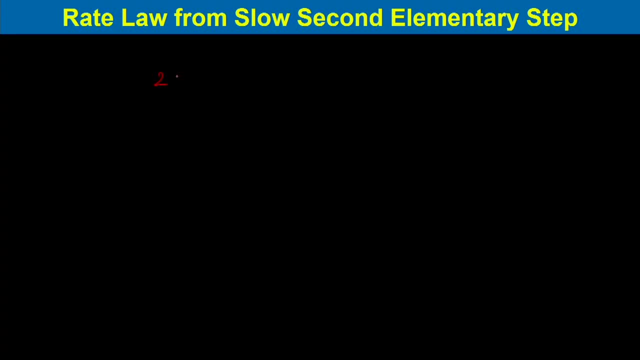 if we consider twice N O plus oxygen forming twice N O 2, the rate is K, concentration of N O square or to the power 2 and concentration of oxygen. So in this case the mechanism we can propose as N O reacts with oxygen form, N O 3, N O 3. 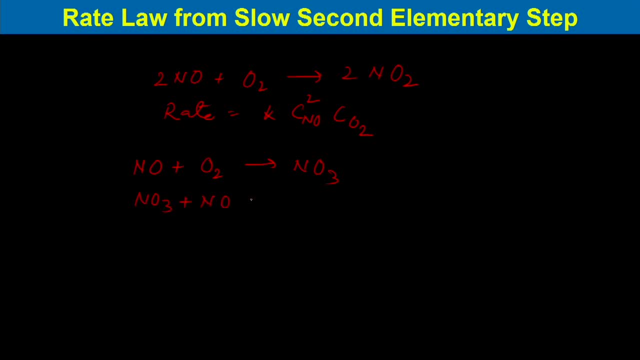 plus N O form twice N O, 2.. So if we sum it up, so this will cancelled out and we will have twice N O plus oxygen forming twice N O, 2.. So this is the overall reaction. So from here, the slowest step is the second step and this is fast. So the rate of reactions: 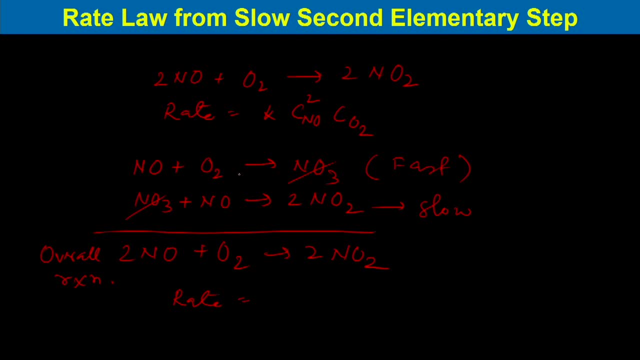 we can write. so this reaction- the first reaction is considered to be the equilibrium reaction and hence this is rate- is written as K 2 into K. equilibrium concentration of N O square concentration of oxygen which is equal to K into concentration of N O 2 square into.